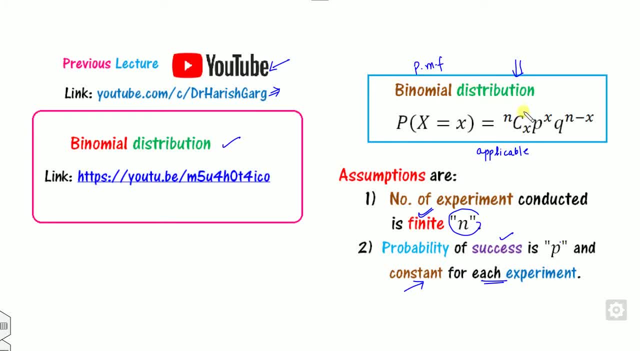 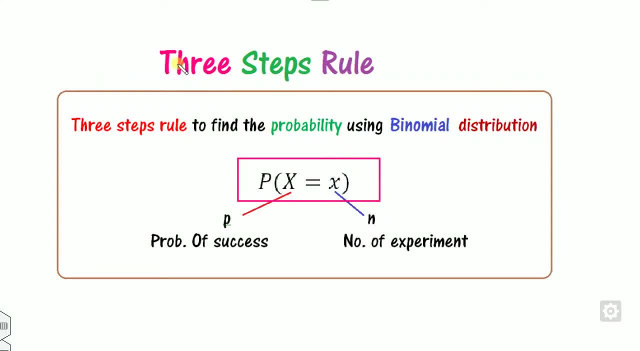 Once these two conditions are satisfied, then you- only you, can apply this binomial distribution. So in this lecture we will see how you can solve the problem. I will follow these three steps Rule. the first step is you have to write everything in form of the probability: X is equal to something. 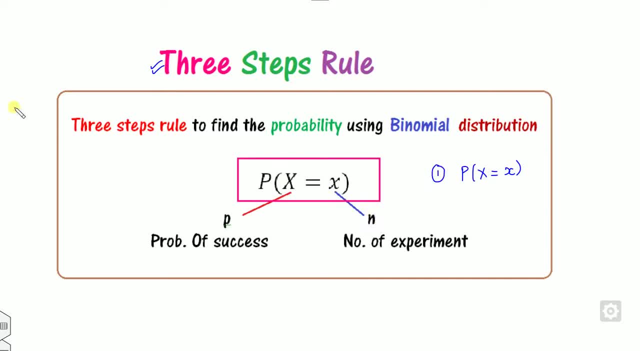 This is my step number one, Since in the binomial distribution there are how many unknown parameters are there? There are two and P. So then my step number two is: you have to find the value of n, which always give from the right hand side of the equation. 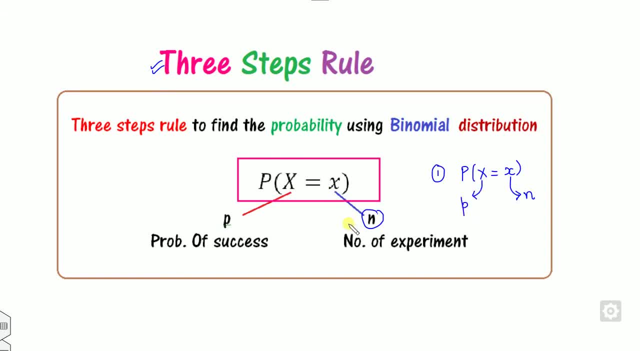 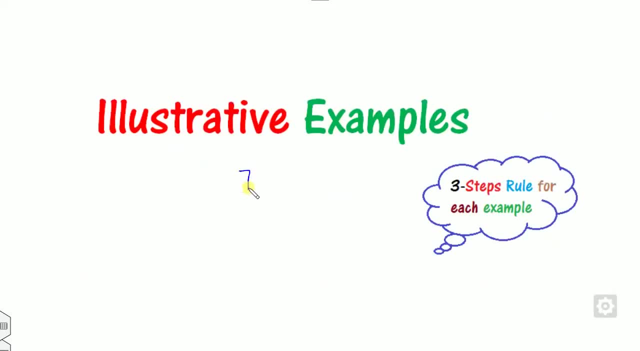 It will give you the n and from the left hand side, it will give you the value of P. That is the probability of success. So, based on this, we can try to Solve the several examples I will consider here in this video, that is, the seven. seven examples are there and each problem will be solved with the help of this three step rule. 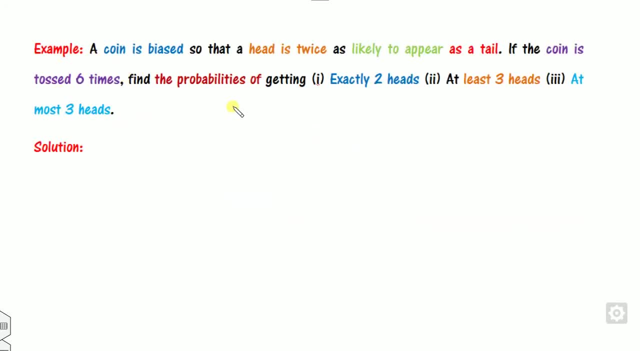 So what is the meaning of that? Look at this statement First of all. instead of reading the line, you have to read first, from this to the first full stop. What is the meaning of that? A coin is biased. The head is twice as that of the tail. 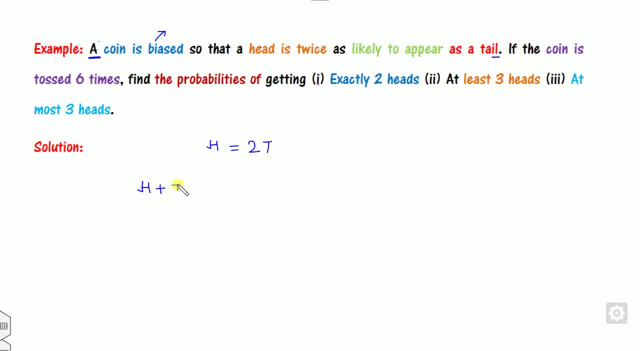 So this is a full stop. So what is the meaning of that? It means we know head plus tail. So if you substitute the value of this, so what you get you can get. the probability of that tail is one by three. Therefore, what is the probability of the head? 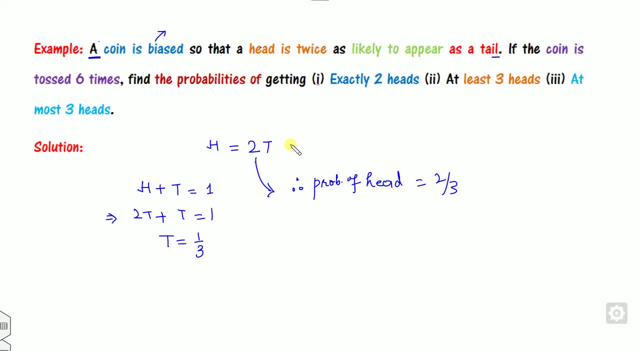 So you can substitute the value of here It will be two by three Now, if the coin is tossed six times. so it means my n is my six. Now what is the first part? Exactly two heads. How you can write in terms of this: 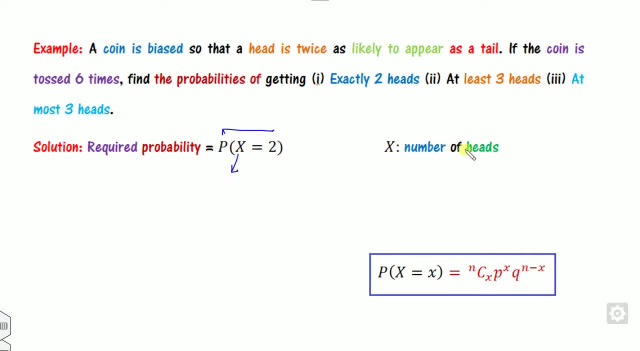 This is the way: exactly two heads. What is the meaning of this? This is number of the head. What is the minimum number of the head you can obtain? What is the maximum number of the head you can obtain, Since the maximum number of the head obtained is six? 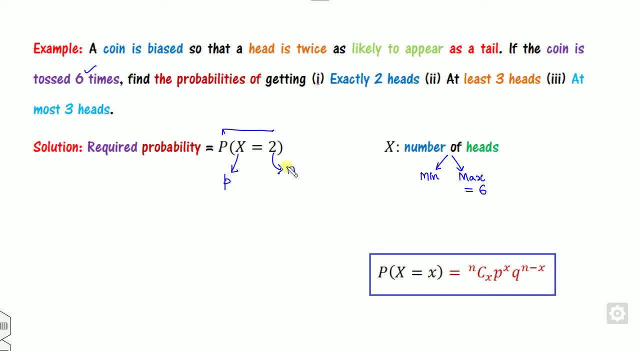 So remember, this is my step number two. This is the n, This is a p. So what is that? This right hand side is the maximum number of the head. So what is? the maximum number of the head is six, So n is my six. 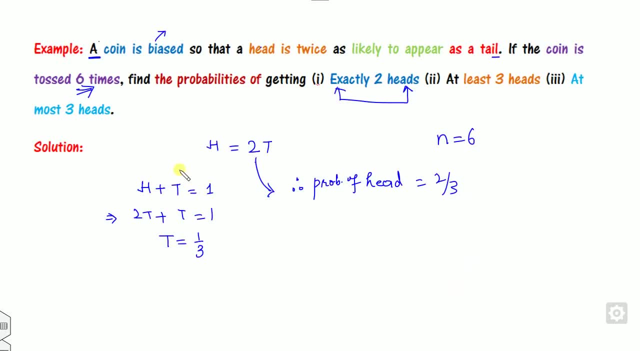 What is the p? is x. What is x is head. What is the probability of the head We have obtained as two by three. So, therefore, what is the p is my 2 by 3. so once you are finding this p and n, and this n is my finite. 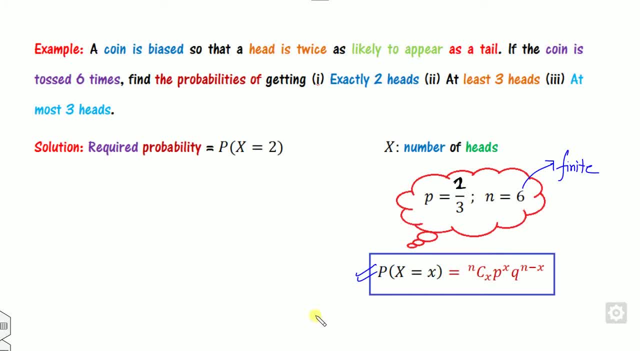 so therefore you can apply this binomial distribution. remember, n is finite, then only you can apply. so what is that now? n, you have 6, x is my 2. you can substitute the value here, you will get ncx. n is my 6 p. so what is the q? q is nothing but my 1 minus p, so that is 1 by 3. 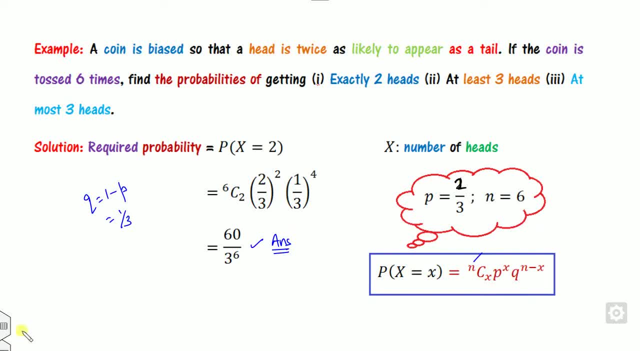 so, after solving, you get the required answer. look at the second part, how you can write. the first step is how you write the probability, something at least three heads, so you can write like this way, at least greater than three. again, what is the x is number of the head. so 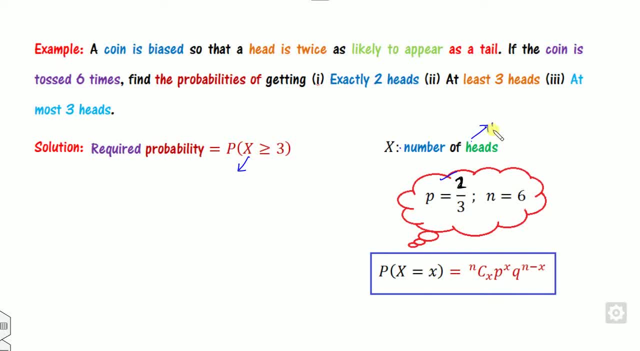 probability is again 2 by 3. what is the maximum number of the head? is my 6? again 6 now, since this is a discrete, so it's equality. so how you can write that? either you can write like this way: x3 plus x4 plus x5 plus x6, because xn is my 6.. Otherwise, instead of them you can also write like 1 minus. 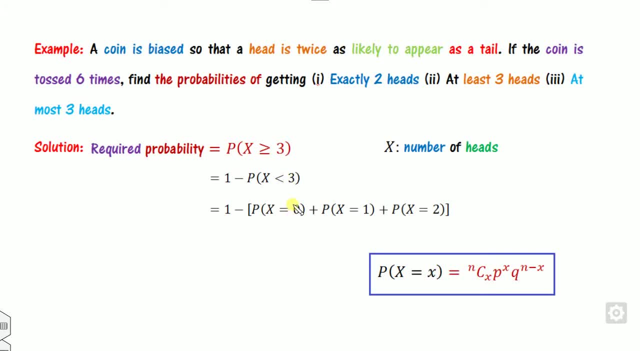 of x less than 3.. And since it is a less than 3, so you can write 0,, 1,, 2.. So, after substituting the value of x, apply the binomial distribution, for here This is nc0 and cx, and so on. After, 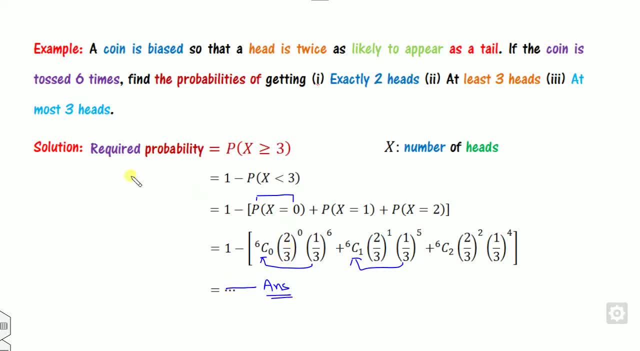 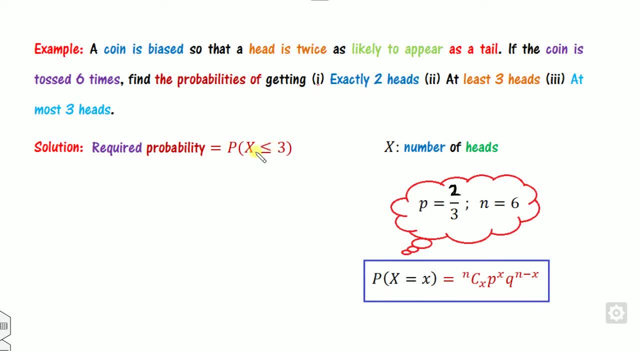 solving, you get the sum answer. that is, the requirements. Look at the third part. Add the most 3 heads. Add the most means there is a maximum. So how you can write: add less than equal to 3? It can be 0,, 1,, 2,- sorry- plus add 3 also. So similarly you can write: 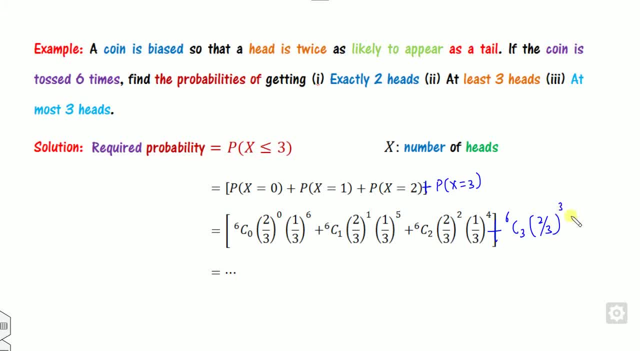 here as 6c3 of 2 by 3 raised to the power 3, 1 raised to the power 3 also. So after solving you get some answers. that is there Again. you may remember that this is my p. 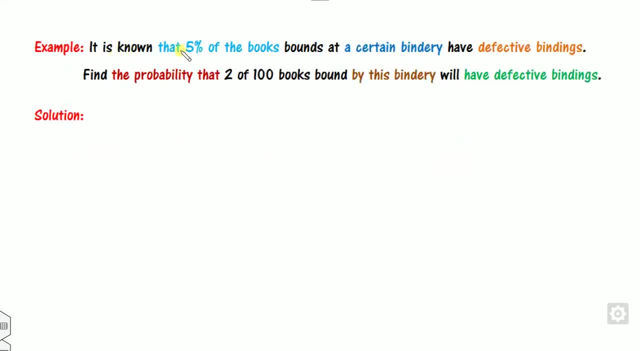 and this is my n. Look at the second example. It is given that the 5 percentage of the books binds are defective. Find the probability that 2 out of the 100 books have defective. So what is your target? You have to find the x is equal to 2.. Now, what is the x here? What is the meaning of? 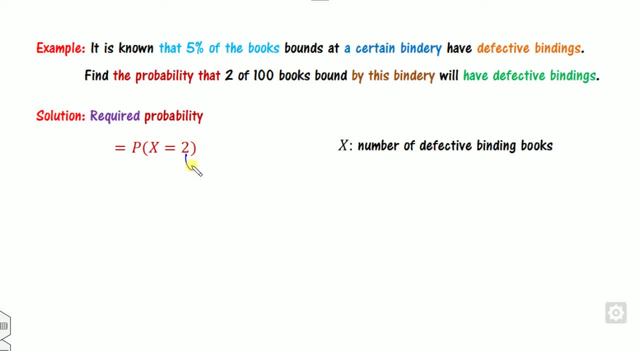 the x. x is nothing but number of the defective bindings. So from here you get the n, from here you get the p. So what is the maximum number of the defective books you can obtain? is 100, because out of the 100 books. So therefore n is my 100. What is the p is Probability. 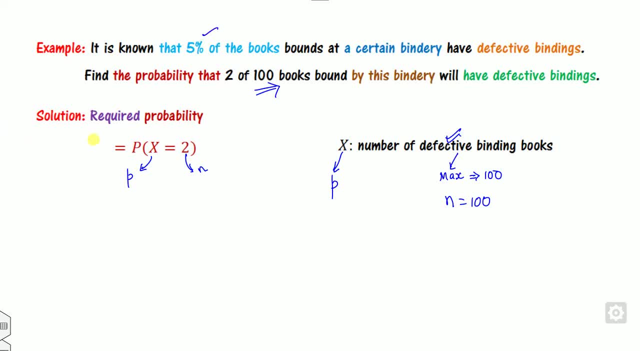 of the x. What is the probability of the x? What is the probability of the x? What is the probability of the defective is 5 percentage. So you can say: p is my, 0.05, n. Now n is my. 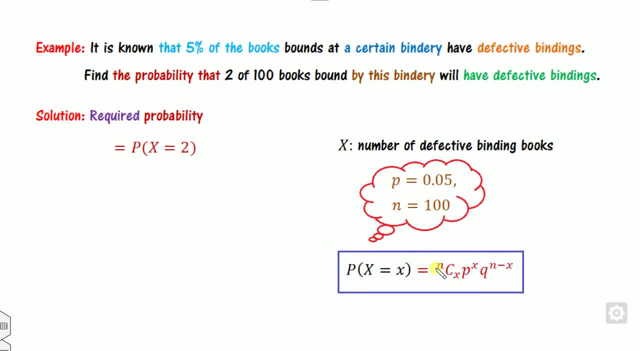 finite number. So therefore you can apply the binomial distribution. So you can substitute here: n is my 100, x is my 2.. You can substitute here: You can see: p is my 0.05,, q is my 0.95. 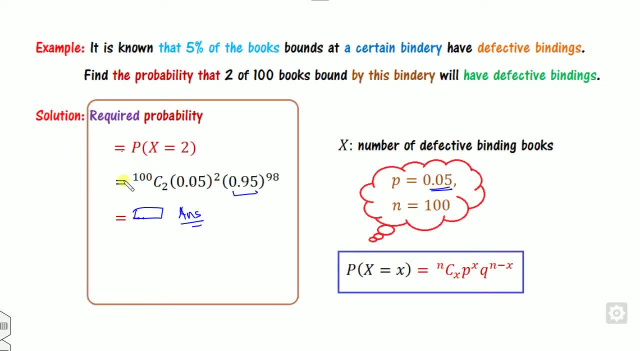 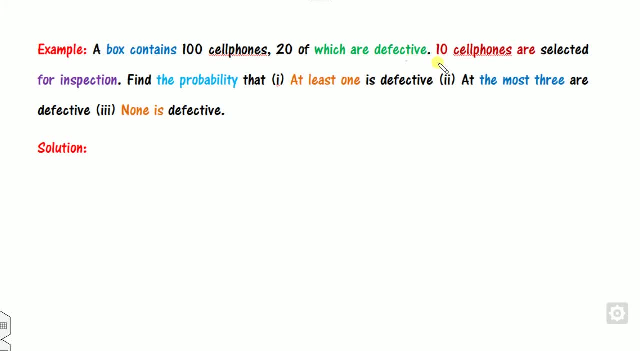 After solving, you get some answers. that is the required answer. Look at that. the 3 step is there. Look at one more example, is there? A box contains 100 cell phones, 20 of which are defective. 10 cell phones are selected for inspection. Find the probability that at least one is. 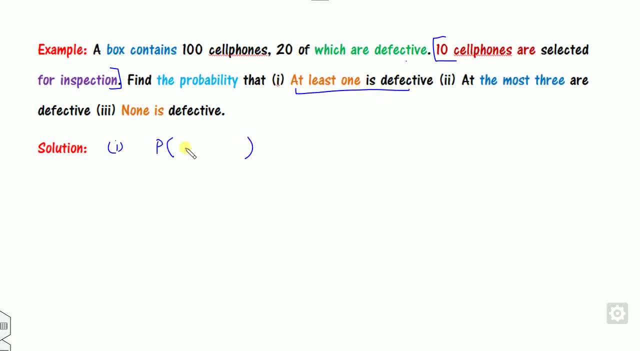 defective. So firstly you have to write: at least one is defective. So this is the meaning of this. What is the x is? What is the meaning of the x? x is my nothing but number of the defective cell phones. What is the maximum number of the defective cell phones? So look, 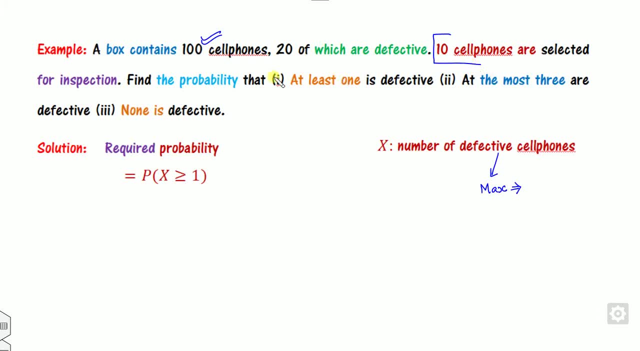 at that, If you have the 100 cell phones, how many cell phones you have picked? that for the inspection is only 10.. So the maximum number of the defectives are only 10.. So n is by 10. And 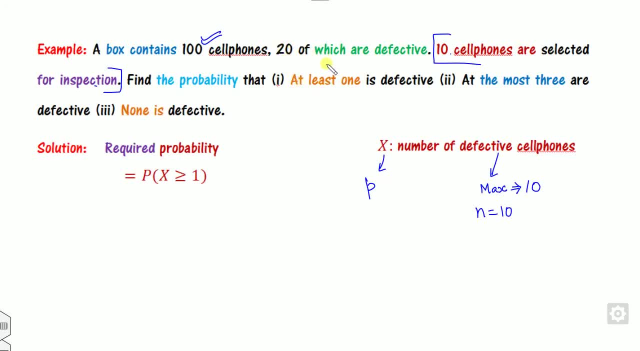 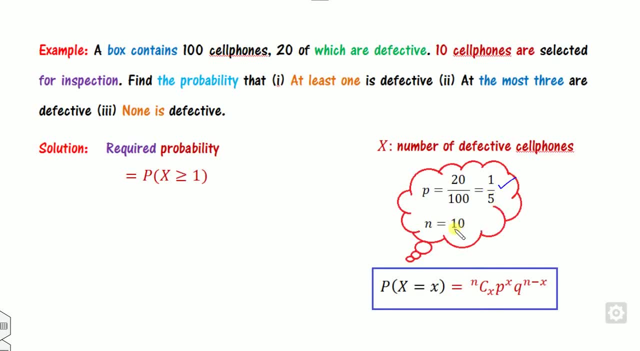 what is the p is Probability of the defective. So what is the probability of defective is there? This is 20 by 100.. So this is my probability of the defective. That is 1 by 5.. Again, n. 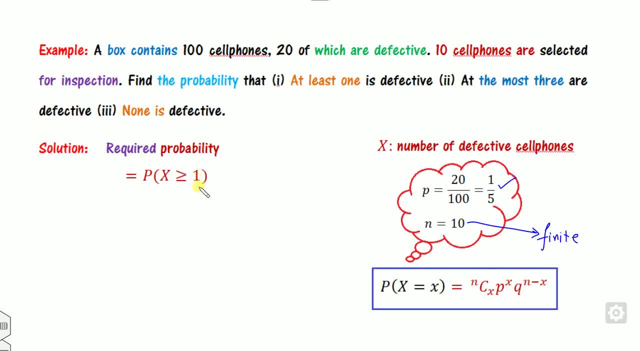 is my finite number, So it is a binomial. So since it is a 10, so you can't write 1 plus 2 plus up to 100. So it is a binomial. So since it is a 10, so you can't write 1. 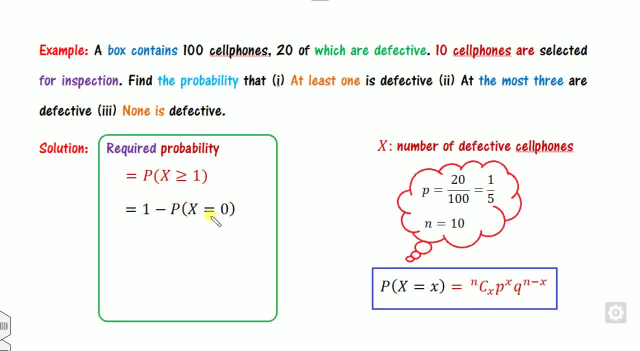 minus 2 plus up to 10.. So instead of them, you can write as 1 minus of this. So apply this as this formula directly. You can solve them. This is the required. Similarly, you can find the second part, At most 3 are defective. So what is the meaning of the at most So? 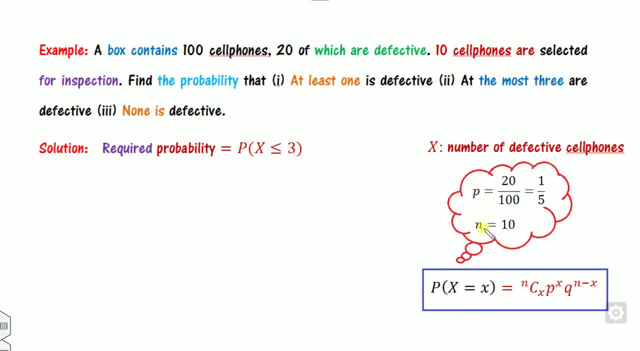 that is less than equal to 3.. Again, p, n is finite, So you can say how you can write this: x less than equal to 3 is it can be 0,, 1,, 2, 3.. Apply the binomial distribution for: 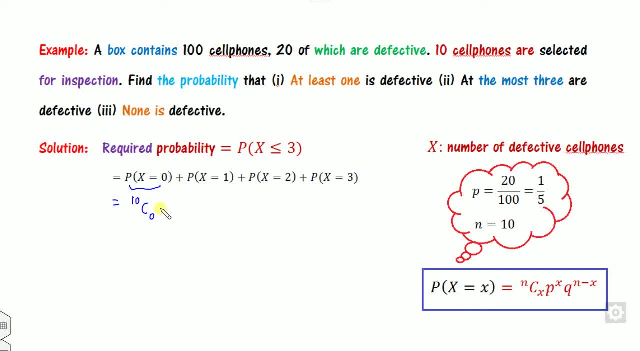 here Again, n is my 10.. So 10 c: 0, 1 by 5 raised to power 0, and what is the k? o is 4 by 5 plus, and so on, You will get: this is the first, this is the second, third, and so on. So after: 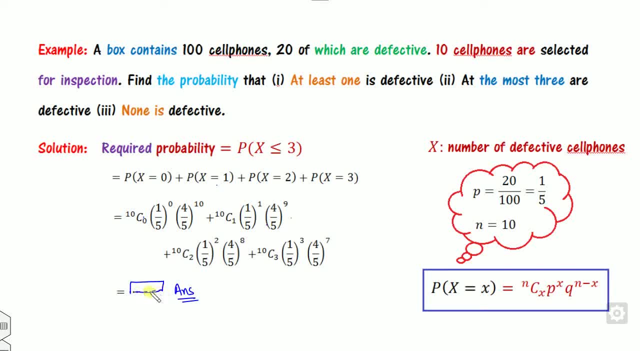 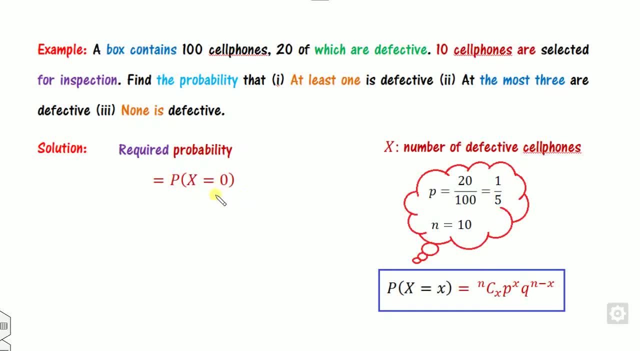 the calculation on your calculator. you will get the required answer here. What is the meaning of them is: none is defective. None means x is equal to 0. Again, since it is already equality, so you can write this as n, c, 0 and so on. 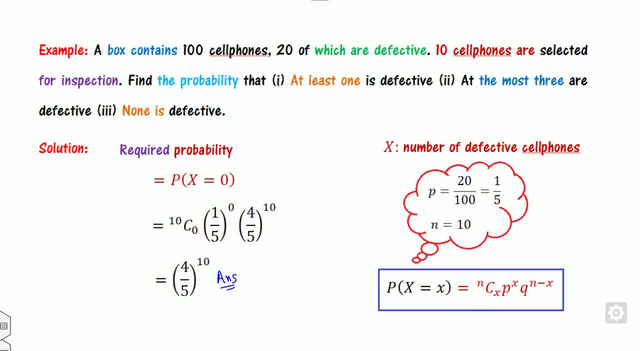 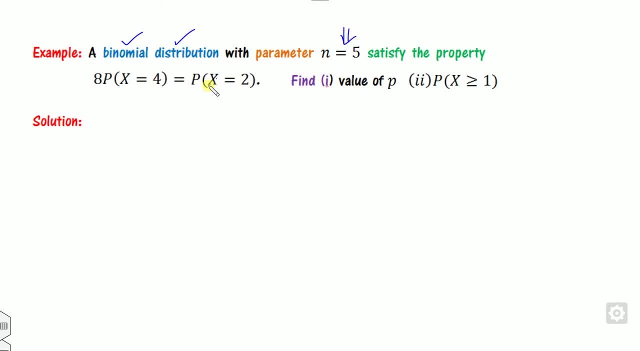 After the calculation you will get here. Look at one more example. is this A binomial distribution with? now, it is given that it is a binomial distribution with finite value of n, and satisfy this situation, you have to find the value of p and this one. So, firstly, 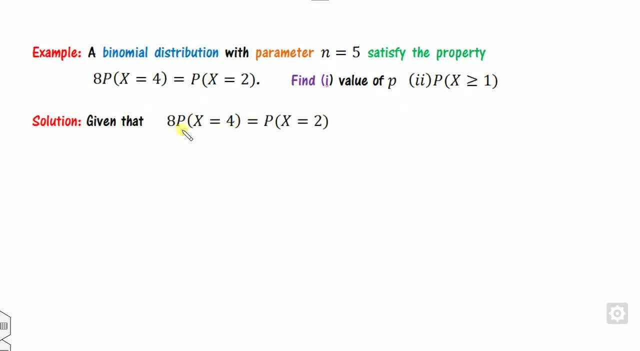 we need a p, So from here how you can expand them. This is a binomial, So you can write this as a binomial expansion and see binomial distribution. and see x- x is my 4, and so on. 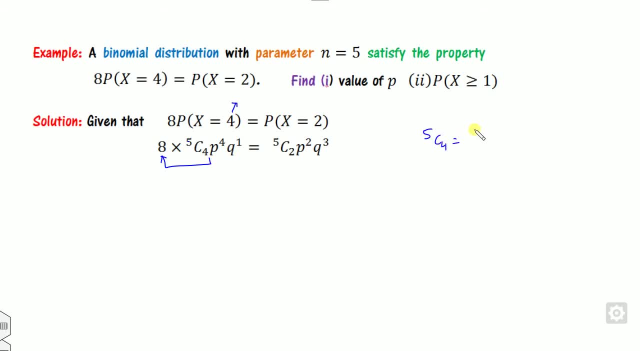 What is that? What is the? This is my 5 c, 4.. This is nothing but my 5 c, 1, or you can say 5.. So this is nothing but my 40 p, 4 q. This is the 10 and so on. So after that you can comment this. What? 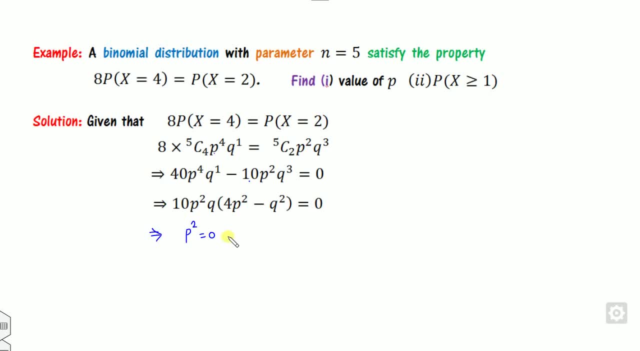 will happen from this: Either p square 0 or q is equal to 0, or 4 p square minus q square is 0.. So once you are solving this, since p and q will never be 0.. So here, So remember. 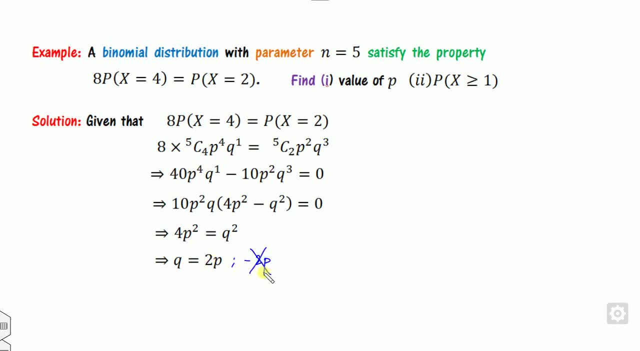 that this will be plus and minus. So since probability can't be negative, so take only as a positive sign p. So therefore now how you find the p is So, since q is my nothing but 1 minus p. So therefore you: 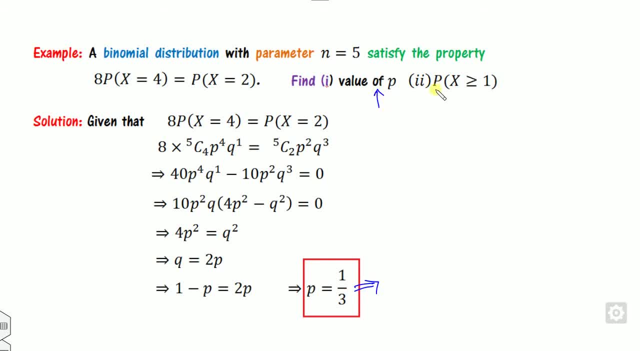 can find the value of p from here. So that's the first part. Now how you find the second part is x greater than equal to 1 means you can write like this way Now: p is my 1 by 3, q is my sorry, p is my 1 by 3, n is my 5.. So you can apply here. So therefore, 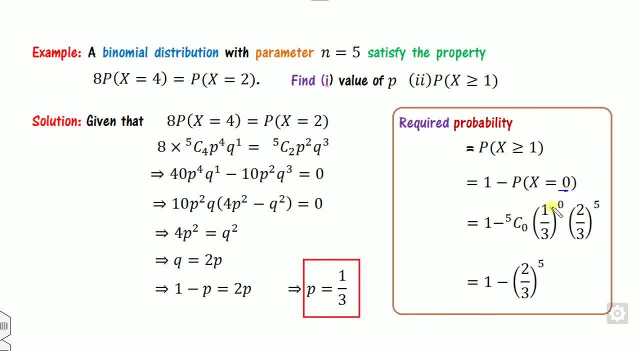 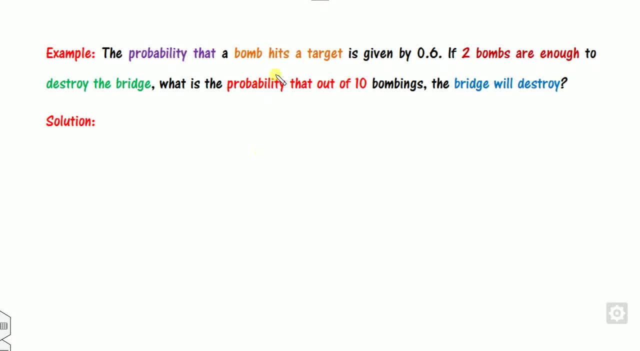 you can find the answer of this: nc0,. x is my 0. So this is the required. If you want to solve this with the help of the calculator, you can do. Look at one more example. is there Probability that a bomb hitting a target is 0.6.. So this is the probability of the hitting. 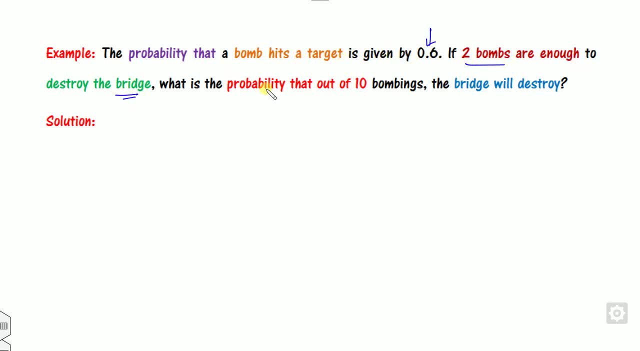 the target, Two bombs are enough to destroy the bridge. Find the probability that, out of the 10 bombing, the bridge will destroy. So when the bridge will be destroyed? So since two bombs are enough, So what is the meaning of that? 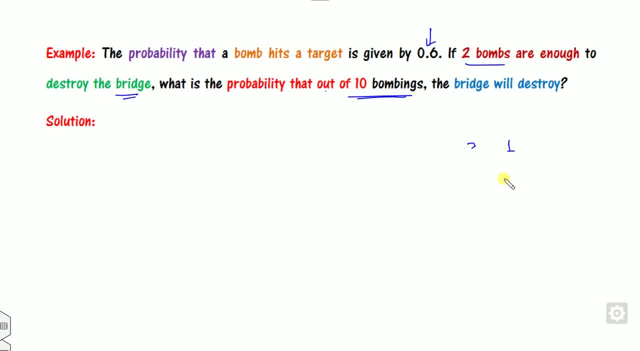 If you throw one bomb, it will not destroy. If you throw the two bombs, it will be destroyed. If you throw the three bombs again, it will be destroyed, and so on. So it means this: the bomb, the bridge, will destroy if you throw at least of the two bombs. And what is the? 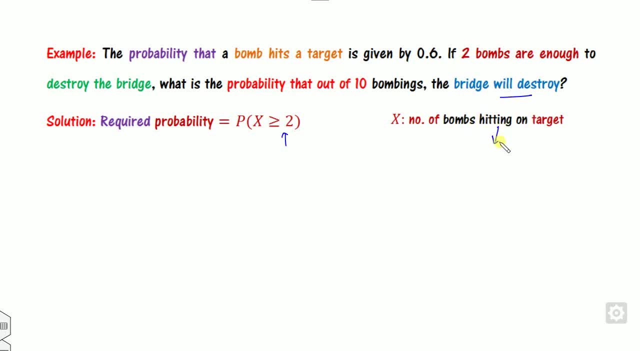 meaning of the x is number of the bombs hitting on the target. What is the maximum number of the bombs you have, Since you have out of the maximum 10.. So therefore, n is my 10.. What is the probability? What is the probability of hitting the target? What is the probability of bomb hitting the 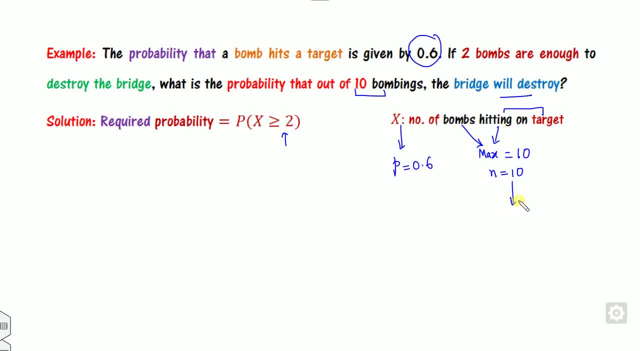 target is 0.6.. So p is my 6,, n is my 10.. So, which is a finite value. So you can apply the binomial distribution again. So it is a greater than equal to 2.. So you can write. 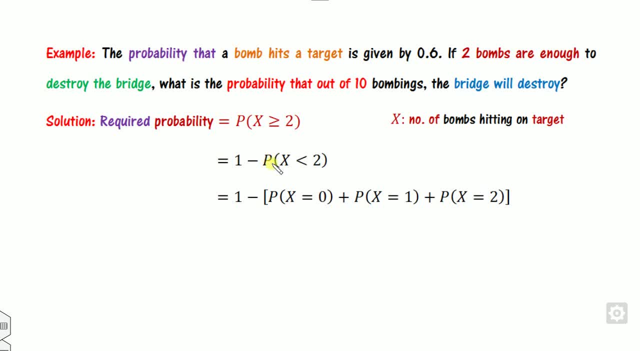 like else, you can write 2 plus 3 up to 10.. Otherwise, you can write as x less than. Since it is strictly less than so, there is no need of this. So once you are finding the binomial distribution, n is my 10.. 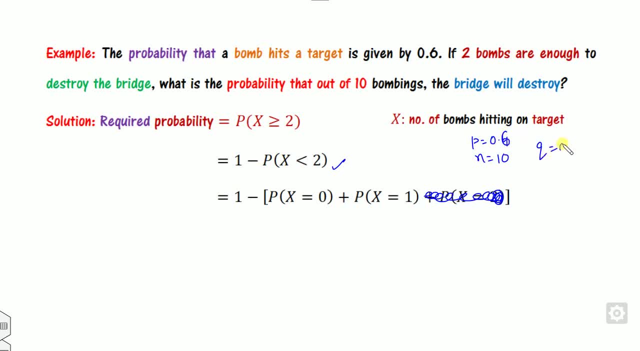 What is the p is my 0.4.. Sorry, 0.6.. What is the q is 0.4.. So once you are substituting the value of this in here, So since this n is equal to 2 is not applicable, So after. 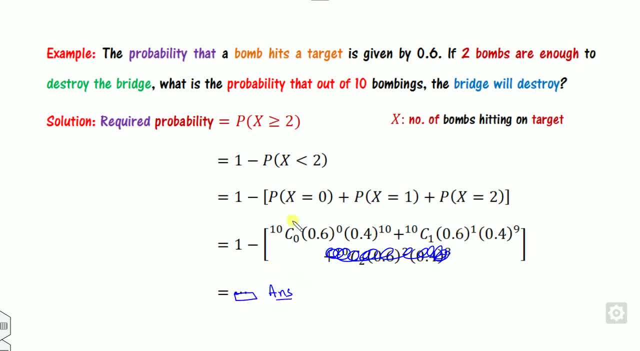 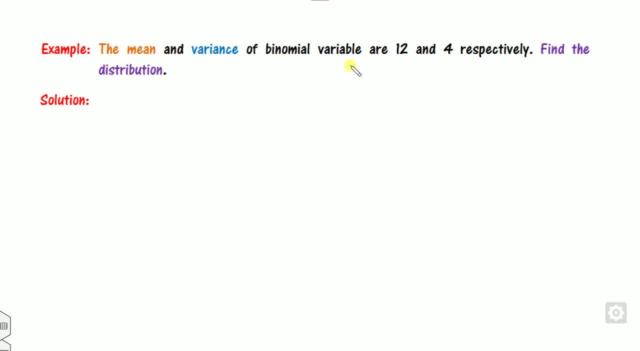 the calculation, you get the required answer. You can solve it with the help of the calculator. Look at the last example. is there? If I say the mean and variance of the binomial variable is given to be here, find that distribution. What is the meaning Now? in this case it. 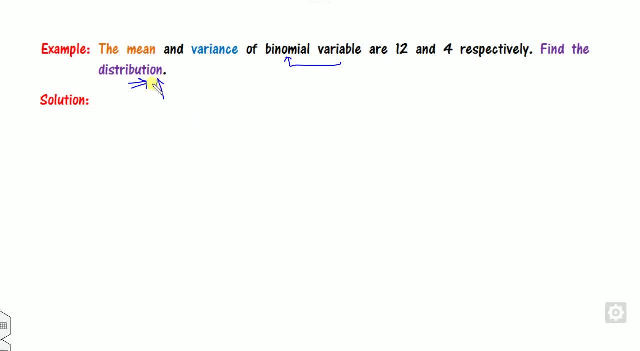 is not given that you have to find the distribution, So you have to find the distribution of the binomial variable. It is given that you have to find the distribution. So, since it is a binomial variable, So your target is to find this one binomial. Look at that How. 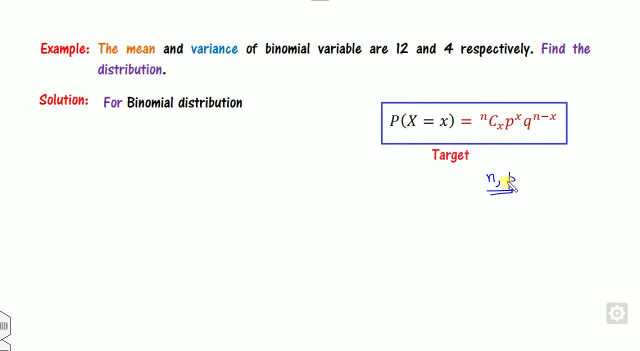 many variables are there. One is the n and second is a p. These are unknown to you, So your target is to find n and p, What is given to you? The mean is given to be 12.. So look at that. the mean and variance are given, And you can see the last video related to the 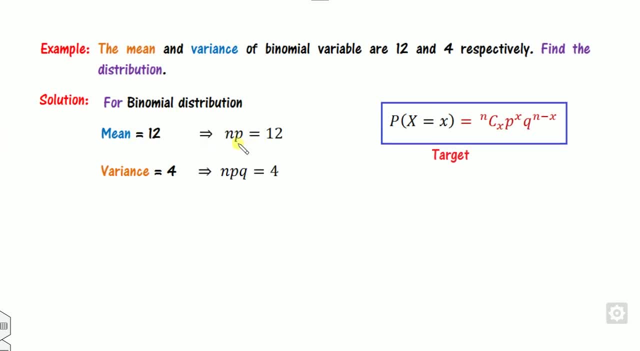 binomial distribution. What is the mean of the binomial distribution? This is nothing but n? p variance is NPKU and it is given. So from these two equations can you find the value of NNP? It's very simple: You can divide them. If you divide, what will happen? NPKU upon NP? 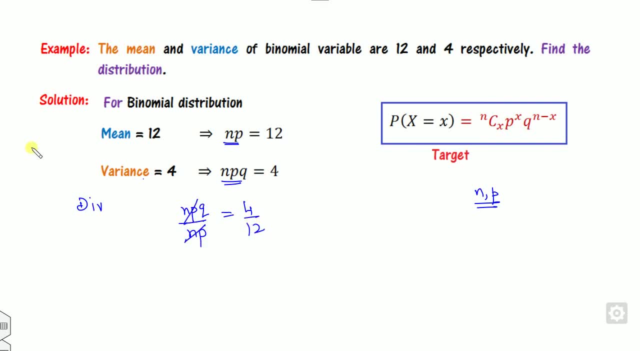 which is nothing but 4 by 12.. So what is that? KU is nothing but 9,, 1 by 3.. Once you know the value of KU, so how you can find: the value of P is 1 minus KU, So this is 1 minus of 1 by 3,. 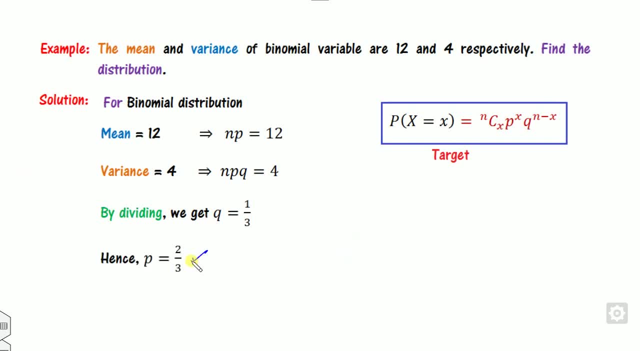 that is 2 by 3.. Once you are finding the value of P, how you find the value of N? So you can use this relation: NP is my 12.. So N is my look at that. N of 2 by 3 is my 12.. So what is the? 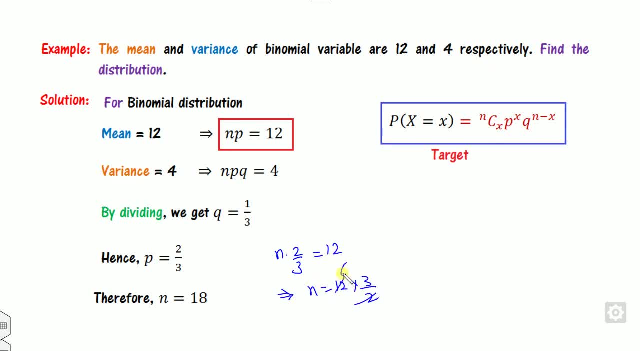 meaning of that. N is my here, So 6, 3 are 18.. Once you are finding the value of N, once you are finding the value of P, you can substitute the value at here. You will get the NCX and 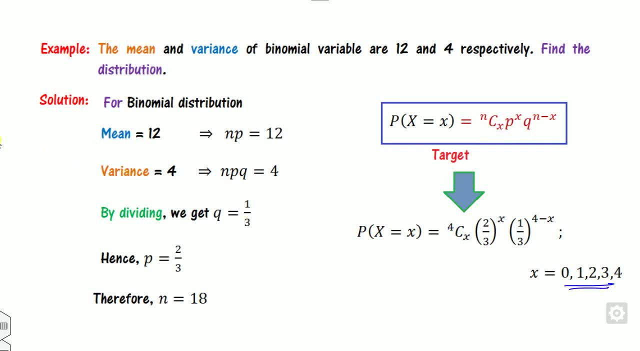 so on. So you can substitute the value at here. You can substitute the value at here. So what is the value of the X? is This one? This is a simple way you can solve this binomial distribution problems. So I hope you can simply learn this simple way to solve this such type of.